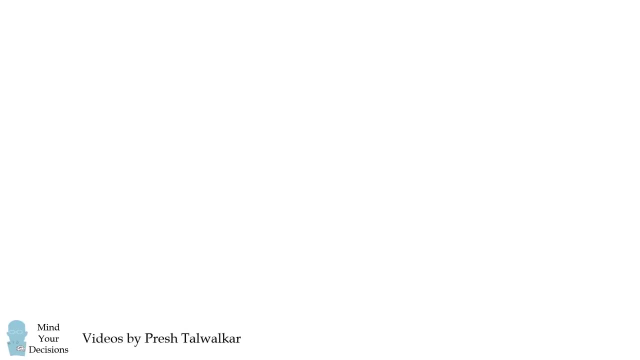 Mind your decisions. I'm Presh Talwalkar. Suppose ABCD is a square, Suppose point E is in the interior, such that angle EDC is equal to 15 degrees and angle ECD is also equal to 15 degrees. Construct EB. The question is to solve for the. 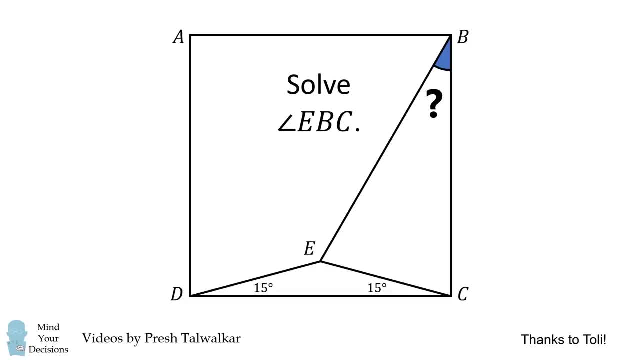 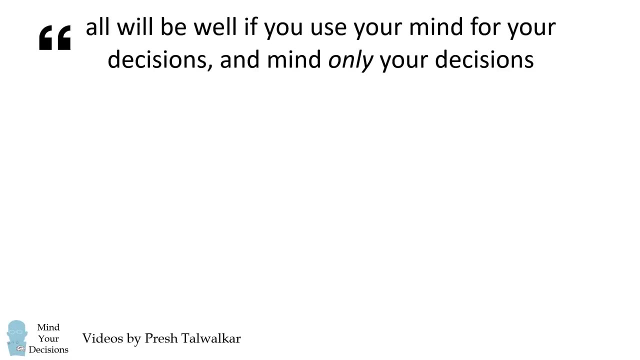 measure of angle EBC. I thank Toli for the suggestion. Pause the video if you'd like to give this problem a try and, when you're ready, keep watching to learn how to solve this problem. I will present two ways to solve the problem. The first uses geometry. 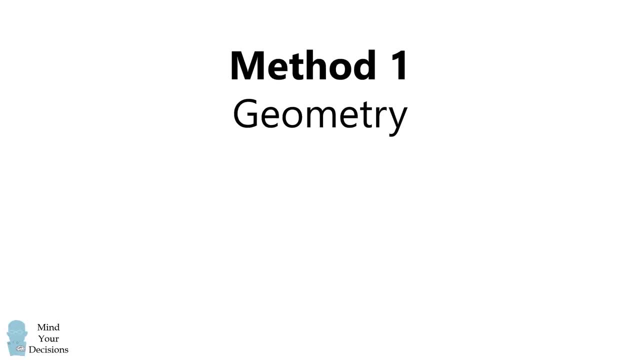 and the second uses trigonometry. Let's get started with the geometry solution. We will first consider triangle EDC. We will construct a congruent triangle alongside BC. Label the point on the interior as F Now, since FCB is equal to 15 degrees and ECD is equal to. 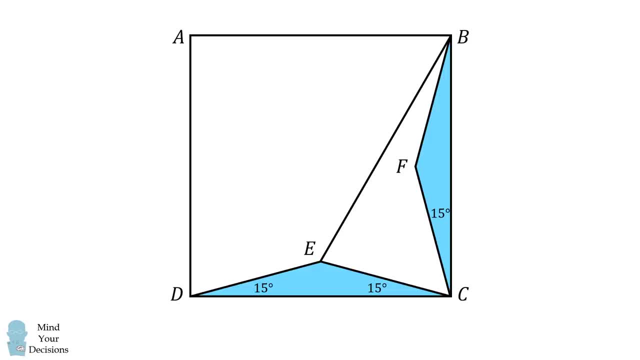 15 degrees and angle C is a right angle which measures 90 degrees, we can conclude that ECF is equal to 60 degrees. Next, construct BC By construction. CF and CE are congruent sides. Therefore we have an isosceles triangle with a. 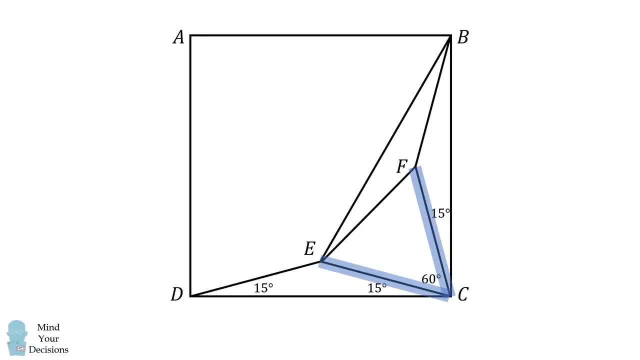 vertex angle equal to 60 degrees. This means the other two angles will both be equal to 60 degrees as well. Therefore, triangle EFC is an equilateral triangle and EF is also equal to EC and FC. From here we will calculate the measure of angle: BFC. 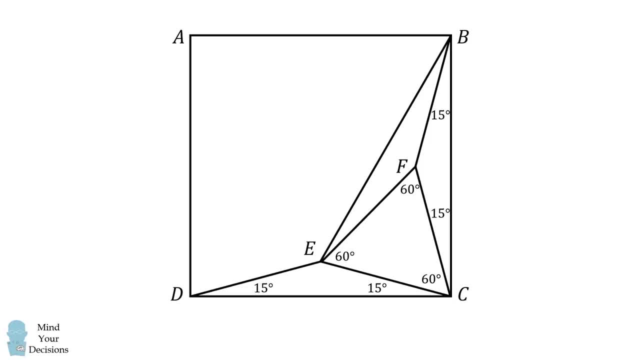 We know that FBC is equal to 15 degrees, so we can calculate the remaining angle in the triangle is equal to 150 degrees. We then have the three angles around. point F must sum to 360 degrees, so we can calculate that EFB is also equal to 150 degrees. We then have the triangles FBC and 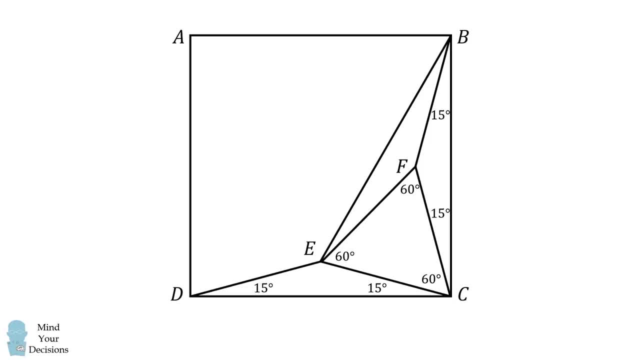 We know that FBC is equal to 15 degrees, so we can calculate the remaining angle in the triangle is equal to 150 degrees. We then have the three angles around. point F must sum to 360 degrees, so we can calculate that EFB is also equal to 150 degrees. We then have the triangles FBC and 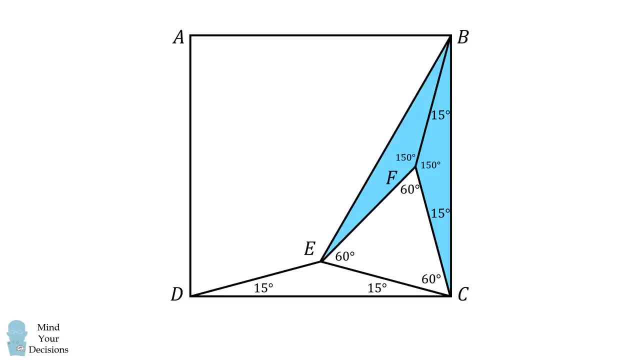 FBE were congruent by side-angle-side. Thus angle FBE is also equal to 15 degrees. Therefore, angle EBC is equal to 15 degrees plus 15 degrees, which is equal to 30 degrees. That's the answer. 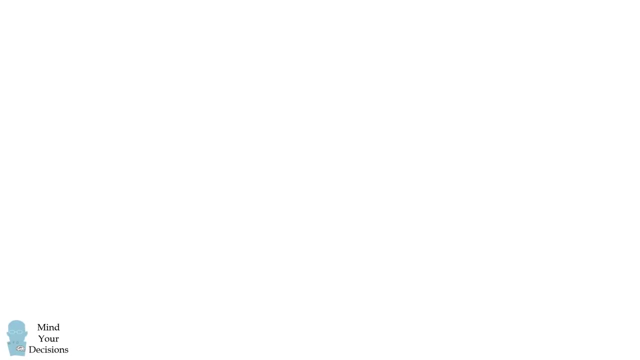 The conclusion shown is a translation of a heads-up. The code is name: housealter, when, when people don't know the denominator. Now let's solve the problem using trigonometry. Suppose ≥ F, ok, esses midpoints. suppose ≥ F is the midpoint of DC. over Dc by 25 and valueYO of nawet Dc by 0 pi over A-B. The right angle, aspirate F and focal angle X is equal to the point AB. the right angle, aspirate F and focal angle AB are congruent by side-angles side. 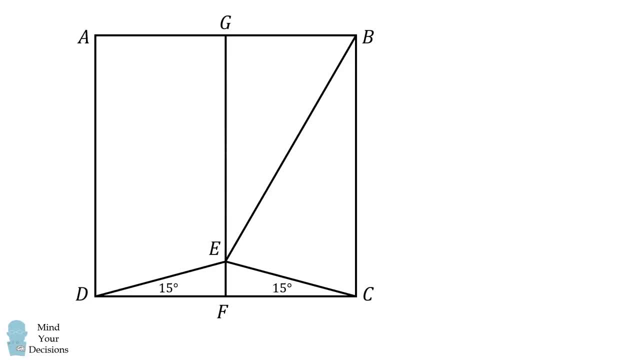 The right angle, aspirate F and focal angle B are congruent by部分 M. FG will be the perpendicular bisector of DC and the perpendicular bisector of AB. Since E is equidistant from the vertices D and C, E will be along FG. 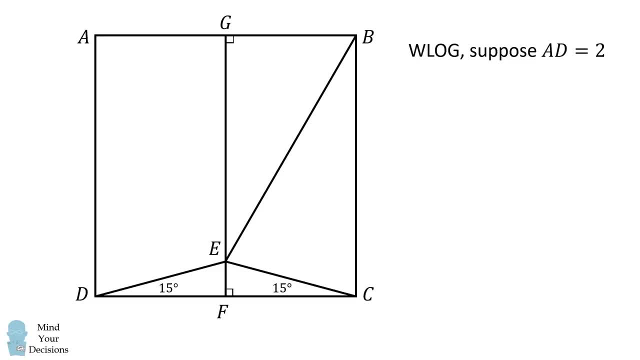 Without loss of generality. suppose the square has a side length equal to 2.. Then FC will be equal to 1, and GB will also be equal to 1.. From here, FE will be equal to the tangent of 15 degrees, which is equal to the tangent. 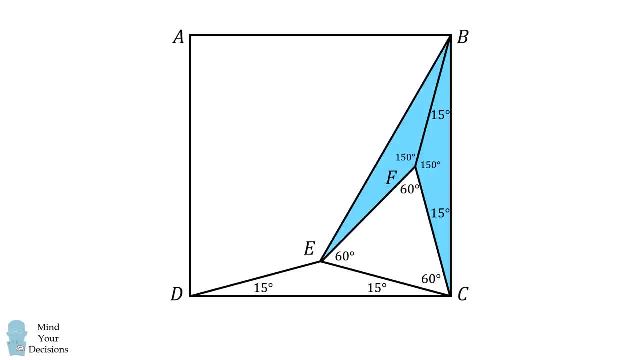 FBE, which are congruent by side, angle side. Thus, angle FBE is also equal to 15 degrees. Therefore, angle EBC is equal to 15 degrees plus 15 degrees, which is equal to 30 degrees, and that's the answer. Let's solve the problem using trigonometry. 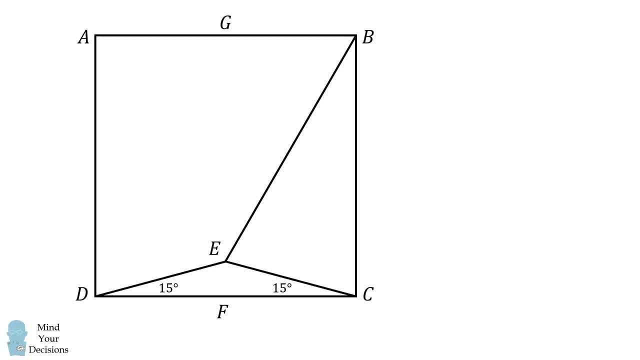 Suppose F is the midpoint of DC and G is the midpoint of AB, FG will be the perpendicular bisector of DC and the perpendicular bisector of AB. Since E is equidistant from the vertices D and C, E will be along FG. 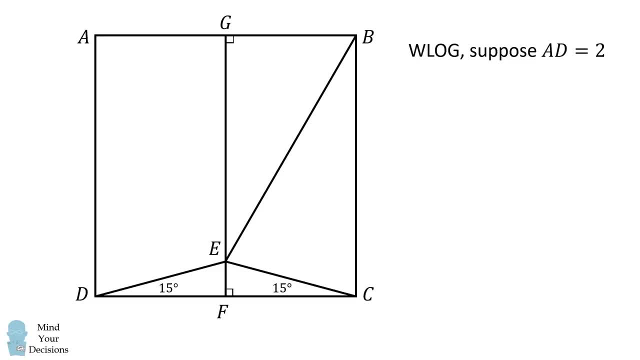 Without loss of generality. suppose the square has a side length equal to 2.. Then FC will be equal to 1, and GB will also be equal to 1.. From here, FE will be equal to the tangent of 15 degrees, which is equal to the tangent. 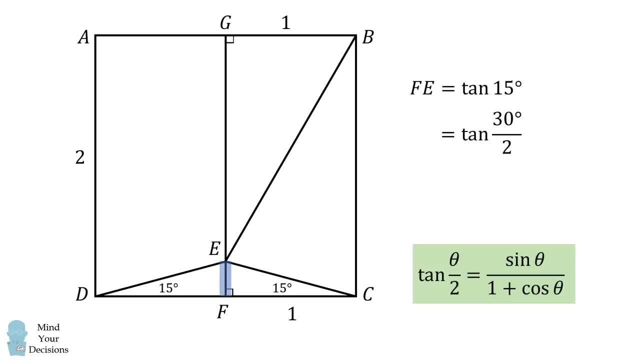 of 30 degrees over 2.. We can then use the tangent half-angle formula. Tangent of theta over 2 is equal to the sine of theta divided by the quantity 1 plus the cosine of theta. We can thus substitute: theta is equal to 30 degrees and it's a routine calculation from. 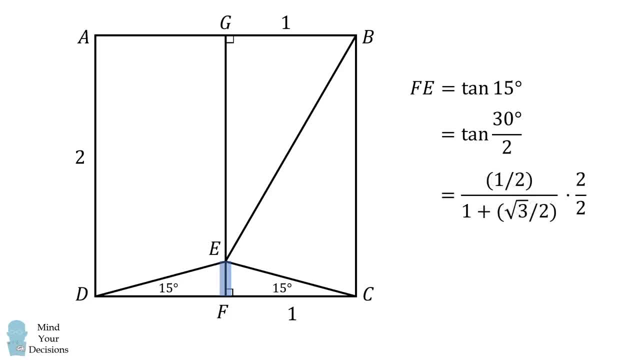 here We merely simplify this fraction, And then we can write this Rationalize it as well. We end up that FE is equal to 2 minus the square root of 3.. Then we can calculate the length of EG. It will be equal to DA minus FE. 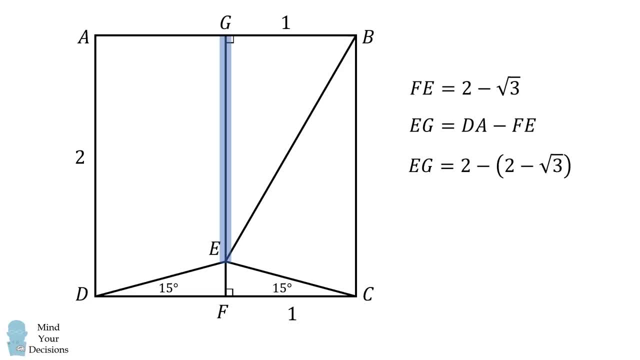 DA is equal to 2.. We've calculated FE. Therefore, EG will be equal to the square root of 3.. From here we will use trigonometry again. Consider angle EBG. We know that it's equal to the inverse tangent of the square root of 3,, which is equal to. 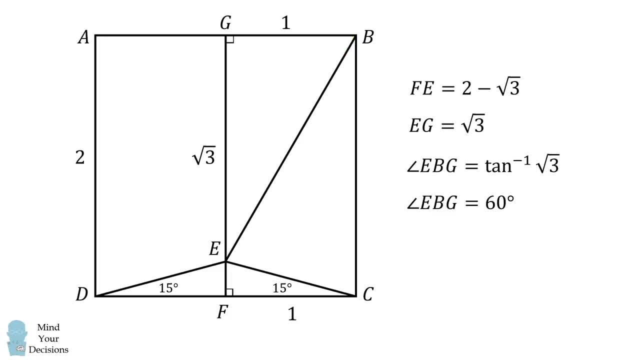 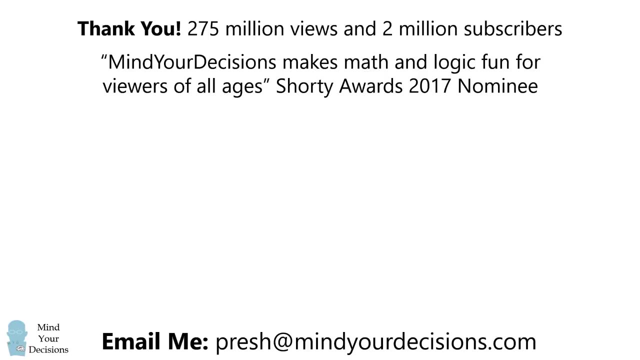 60 degrees, Then angle B is a right angle. Therefore, angle EBC must be equal to 30 degrees, And that's our answer. Thanks for making us one of the best communities on YouTube. See you next episode of Mind Your Decisions, where we solve the world's problems. one video: 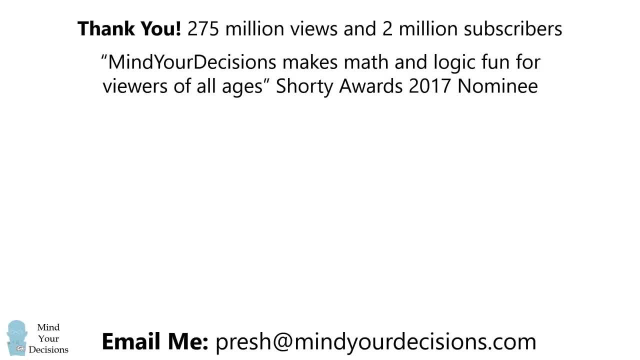 at a time: Bye, Bye, Bye, Bye, Bye, Bye. 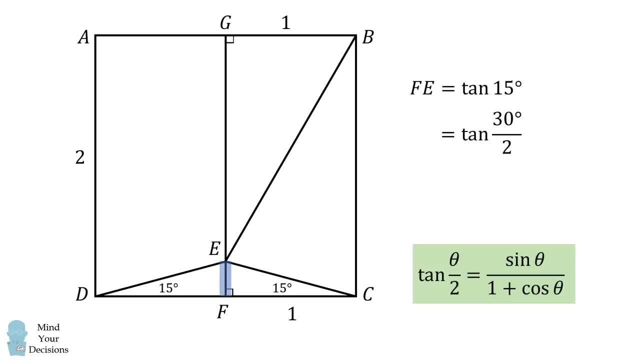 of 30 degrees over 2.. We can then use the tangent half-angle formula. Tangent of theta over 2 is equal to the sine of theta divided by the quantity 1 plus the cosine of theta. We can thus substitute: theta is equal to 30 degrees and it's a routine calculation from. 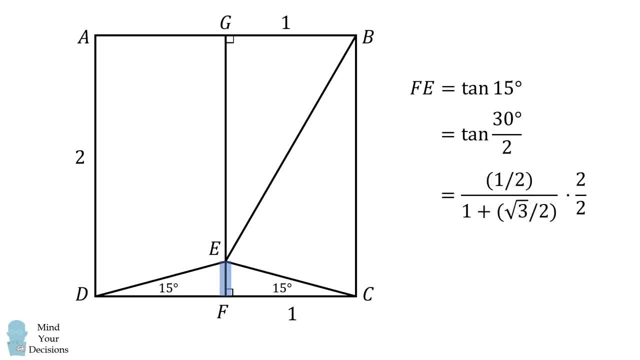 here We merely simplify this fraction, And then we can write this Rationalize it as well. We end up that FE is equal to 2 minus the square root of 3.. Then we can calculate the length of EG. It will be equal to DA minus FE.